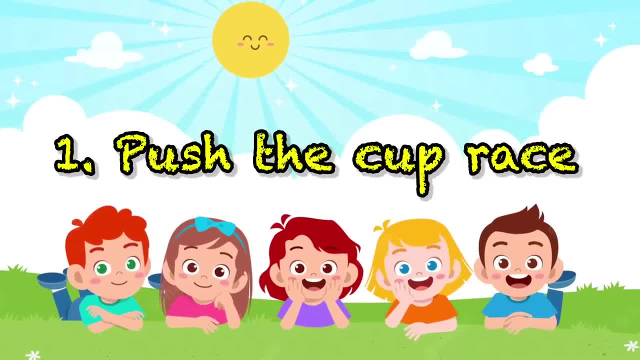 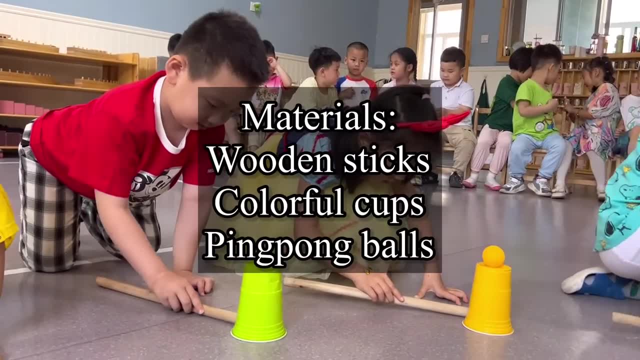 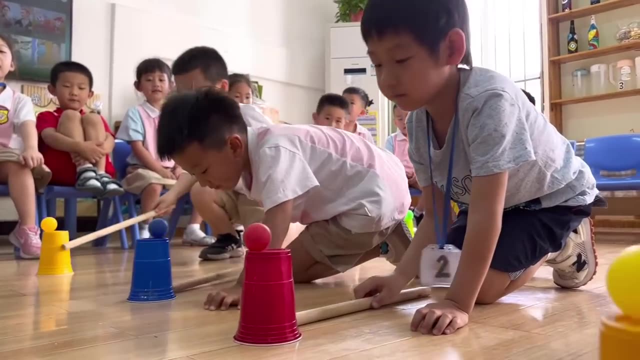 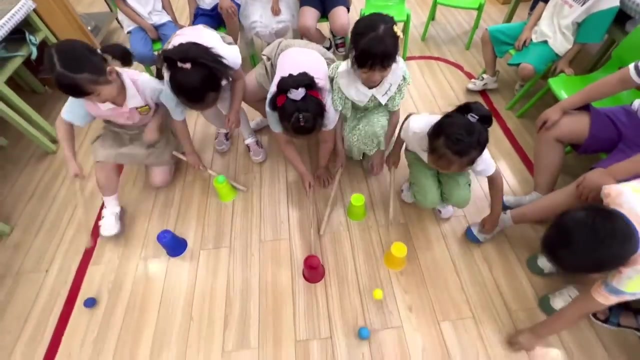 Push the Cup Race- Wooden Sticks, Colorful Cups and Ping-Pong Balls. So all you have to do is put the ping-pong balls on top of each cups and ask the kids to push the cups, using the sticks, towards the flashcards by avoiding the ping-pong ball to fall down on the floor. 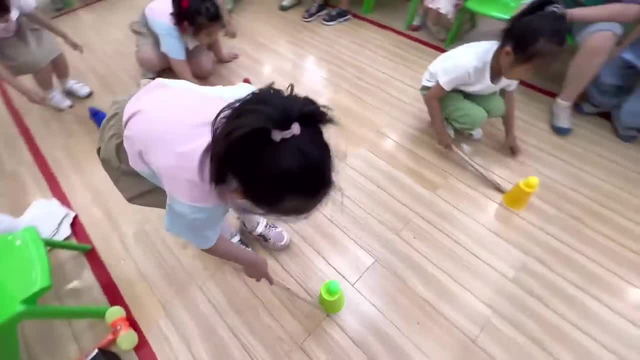 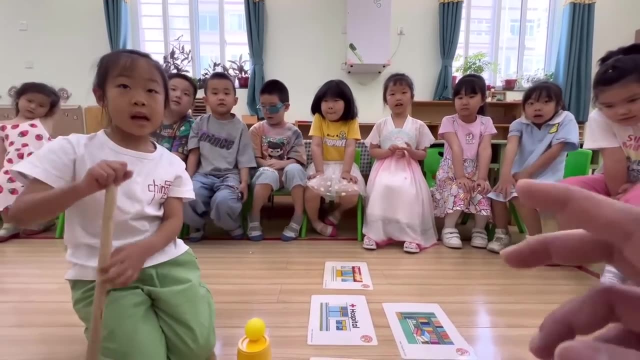 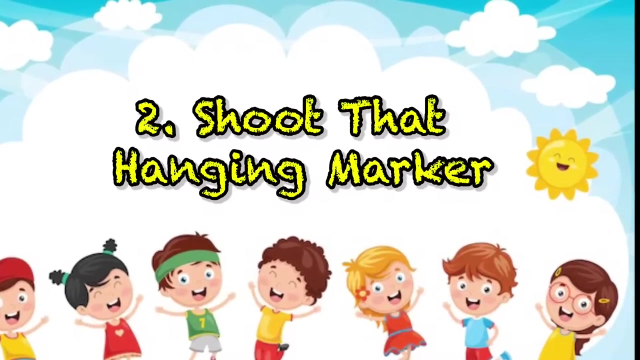 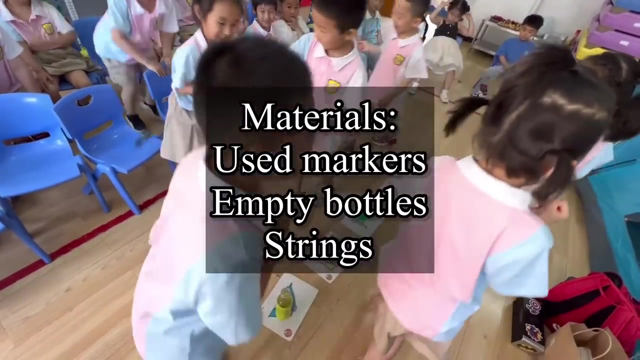 So the first one who reaches the flashcards wins the game And let the kids ask them to. you know. say the words or recite the word. Shoot the Hanging Marker Materials. Use the markers into bottles and strings. There are two ways I play this game. 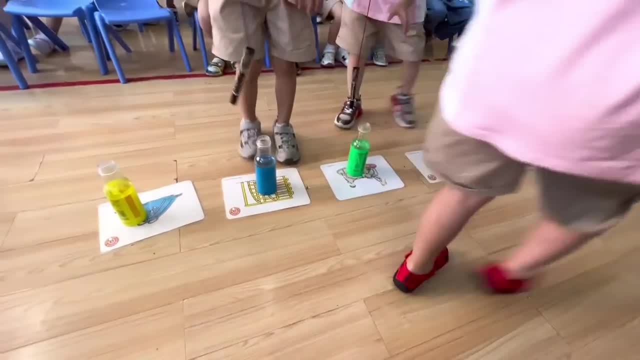 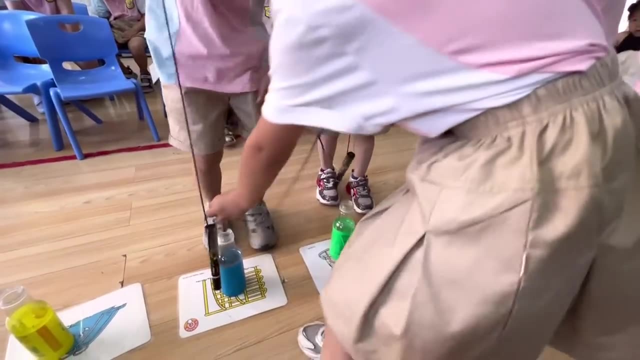 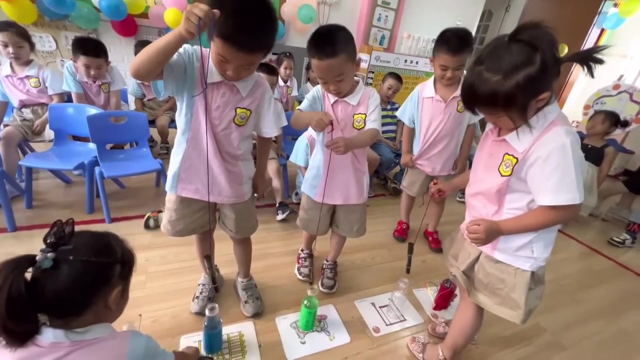 But first I usually lay down the flashcards on the floor and the first option is that I give out the used markers with strings to the kids and then I play the music, and when the music stops they have to shoot the marker in the empty bottle using only one hand. 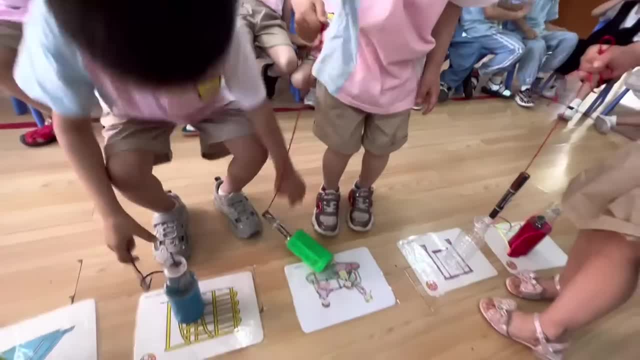 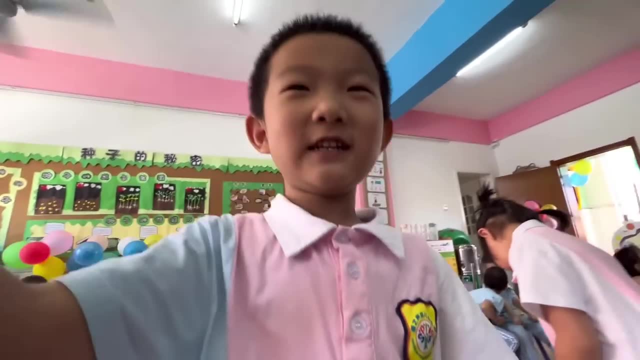 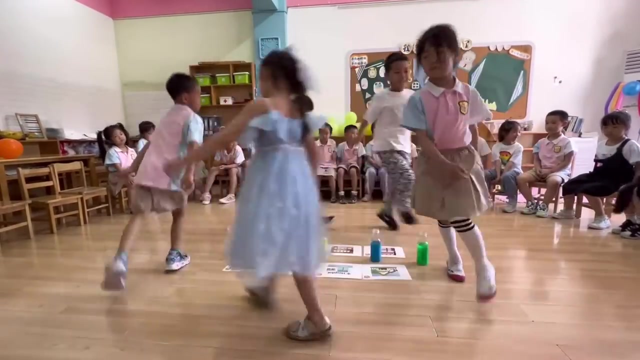 Encourage them not to use the other hand because it wouldn't be that exciting. but you know you can't control the kids, So it's up to you. How do you play, How you manage the game? The second option is that I usually hide the markers with strings. 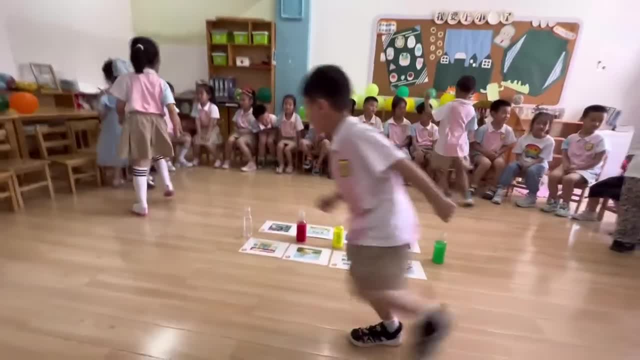 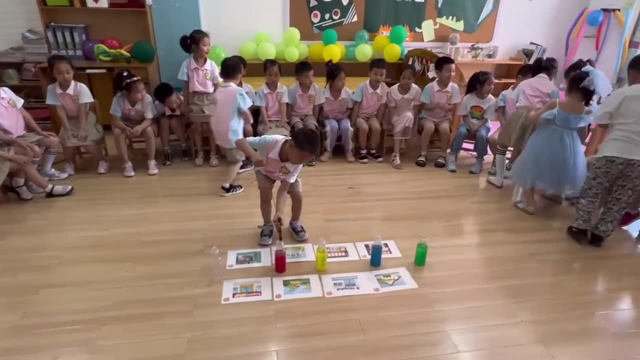 behind or in at the back of the kids sitting, and when the music stops, the players must find one of these markers and then they have to shoot it in inside the bottle and Then they have to say the words. So yeah, that's how I usually play this game. 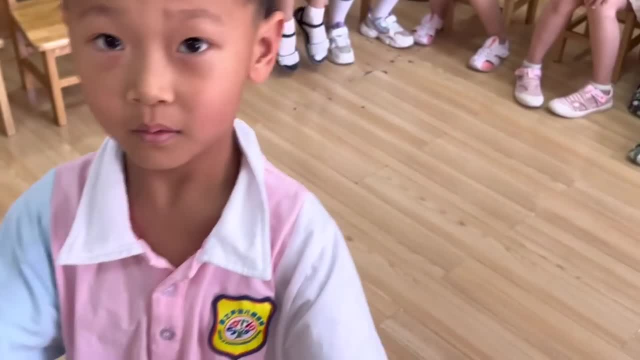 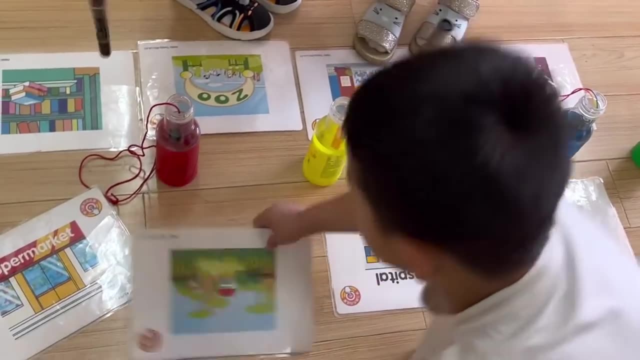 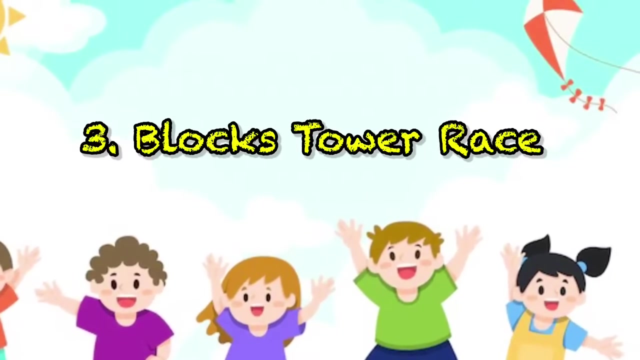 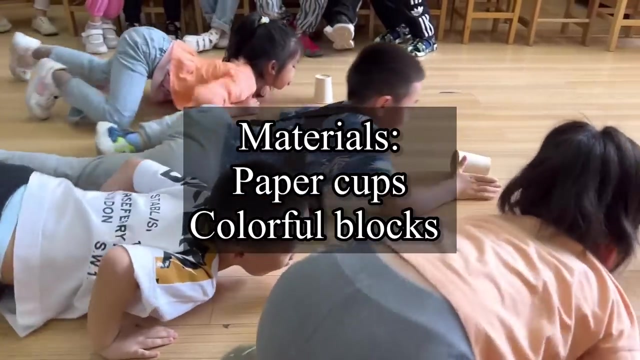 Hi, I'm a little kid. It's super mini kid. Eri, where are you going? I'm going to the park. Good Blocks, tower, race Materials, paper cuffs, Colorful blocks. In this game, you need to put or lay down the paper cups on the floor and 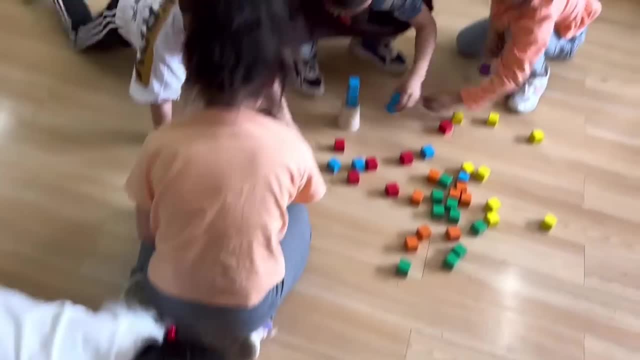 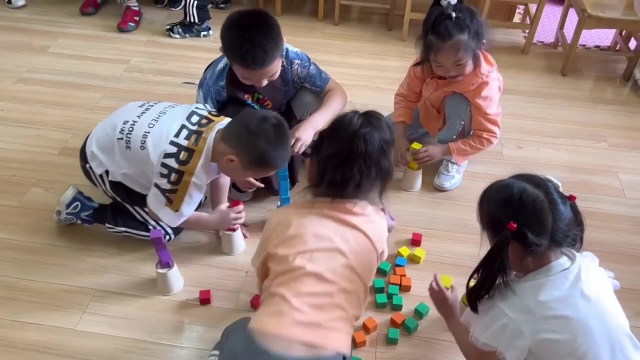 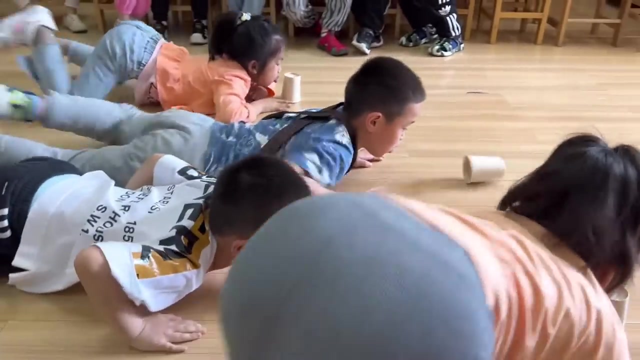 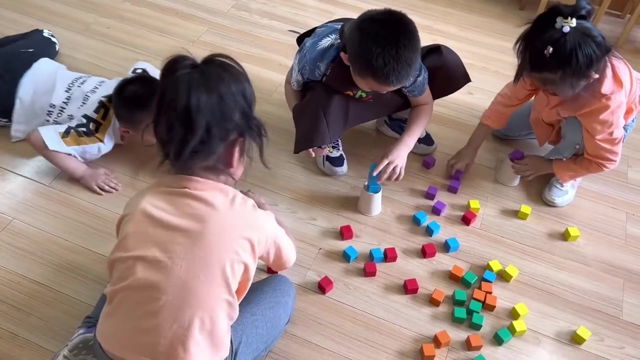 on the other side are these colorful blocks and the flashcards on the other side. so once the materials are all set, ask the kids to blow the paper cups towards the colorful cubes and they have to stack up all those same colored blocks on top of each cup that they have. and once they have made a tower of, 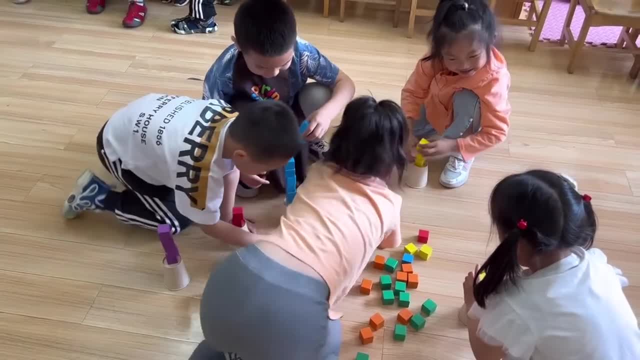 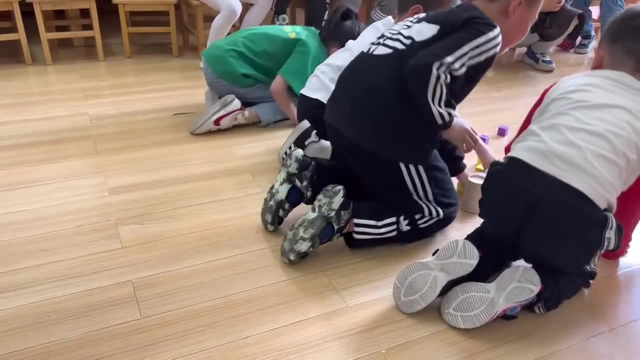 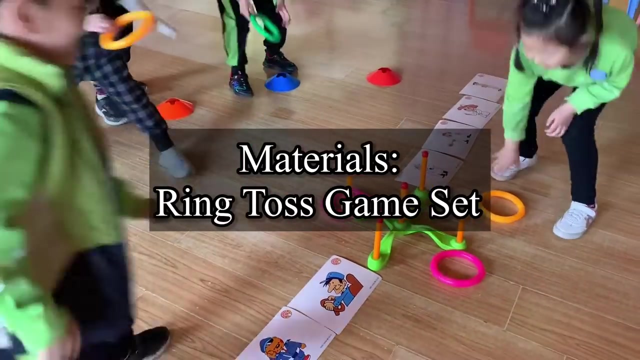 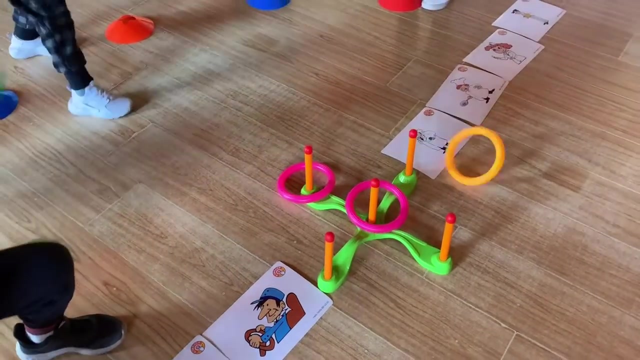 blocks. they have to say the word or the target sentences that you have. ring toss game materials. ring toss game set. this game is called ring toss game set, one of my favorites, and my kids love it too, so it's very interesting and fun to play. so all you 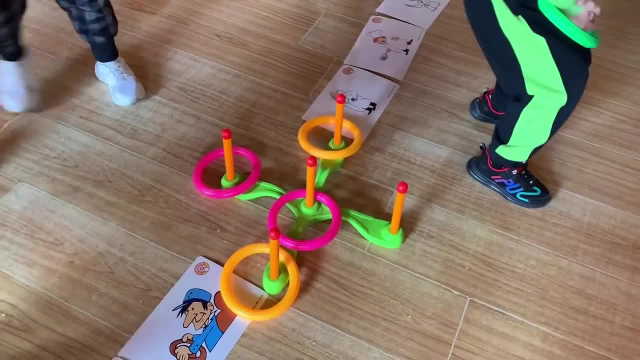 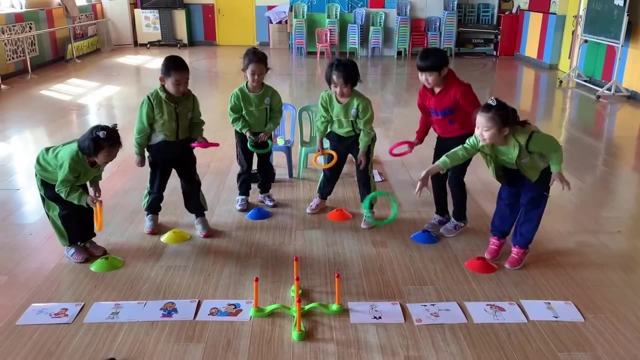 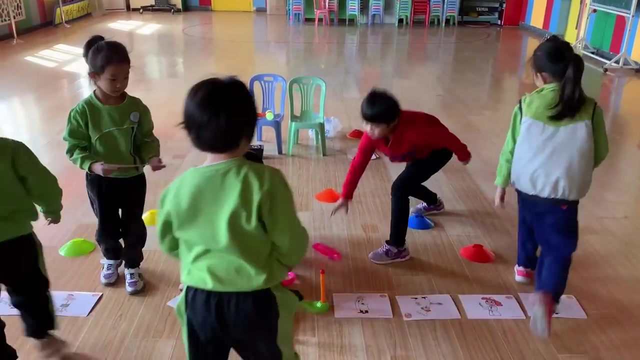 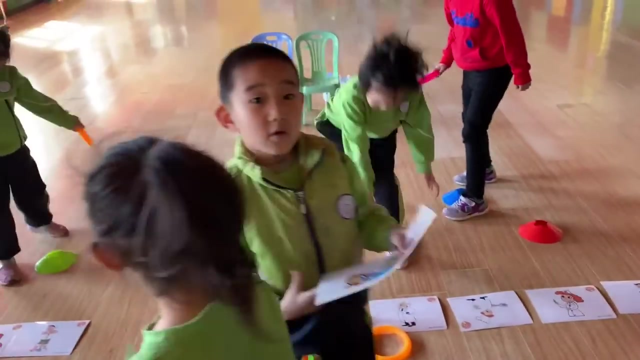 have to do is prepare the ring toss game set in front of the class. you can put markers where the kids should stand and put the ring or the rings in front of them. so you make a go signal and they have to toss or throw the rings together. and once they shoot it on the on the sticks, then they have. 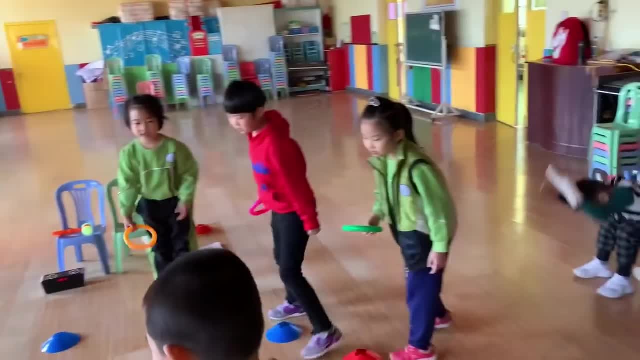 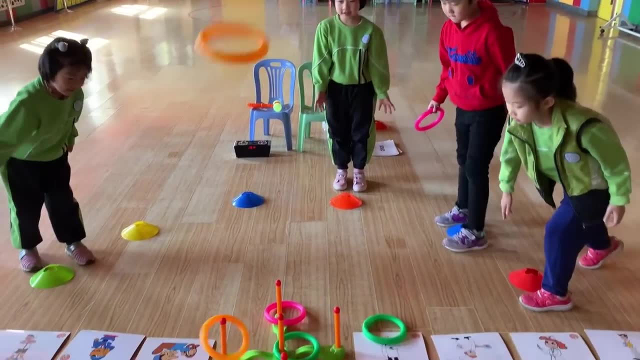 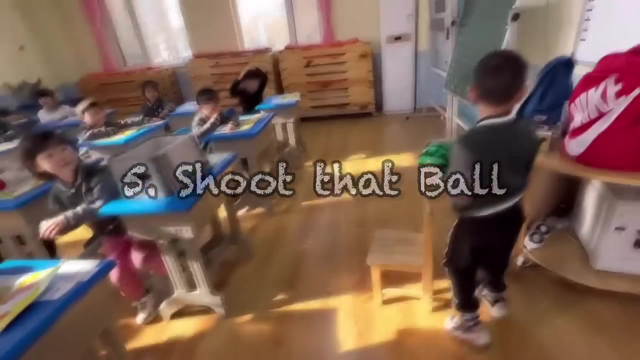 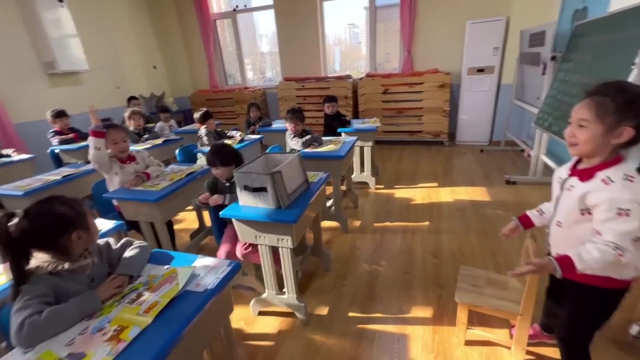 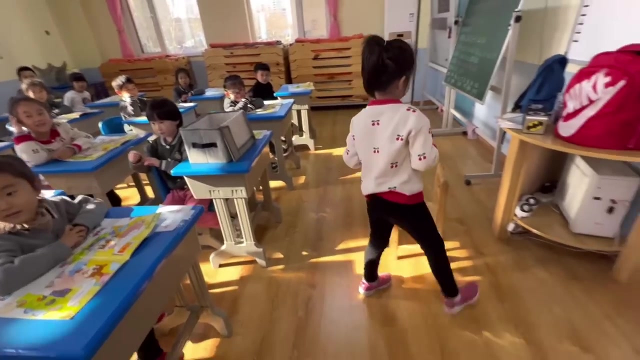 to say the words. you can buy this device or this game. set online. shoot that ball. materials: empty box and ball. this game is ideal for smaller sized class, so all you have to do is put the box on a table in front of the class and also the flash cards or the target words in the box. call out a student and 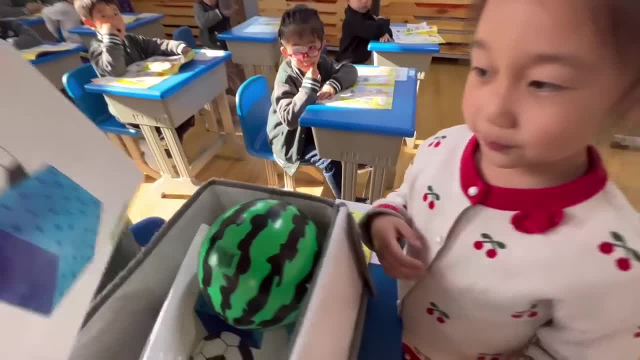 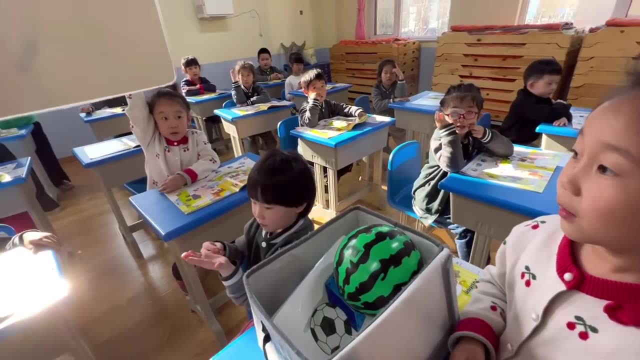 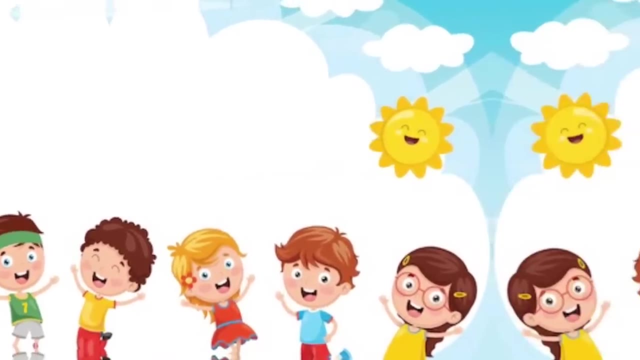 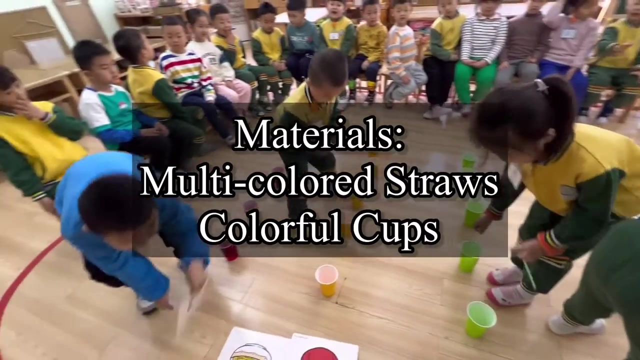 shoot the ball. the student can say or choose the words in the box, or the teacher can can ask the student to recite the words or the sentence study. i'll give you an example of this: materials: multi-colored straws and colorful cups when playing this game. it's short, so i like to put it miniatly. 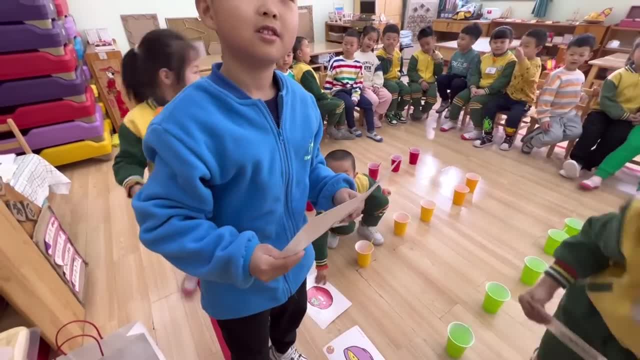 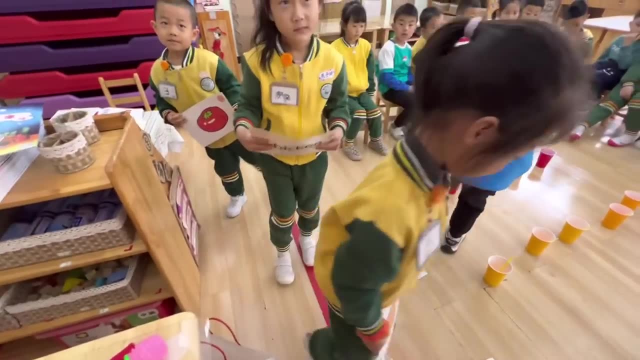 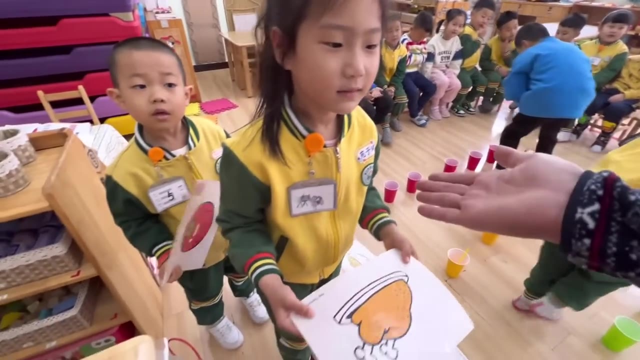 this game needs lots of cups and straws, so all you have to do is line up these cups according to their colors. um, you can line up three cups, uh each uh lines, depending on the time you have in. in my case, I've got plenty of time, so I lined up five cups each. 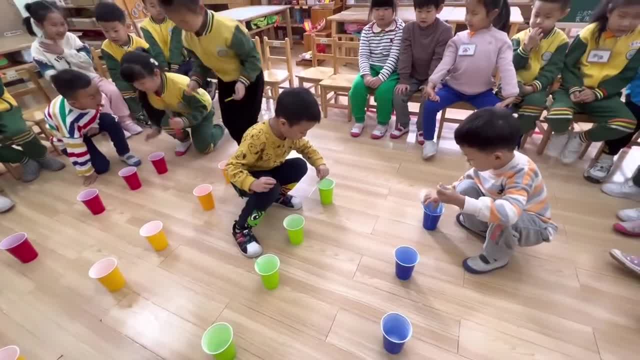 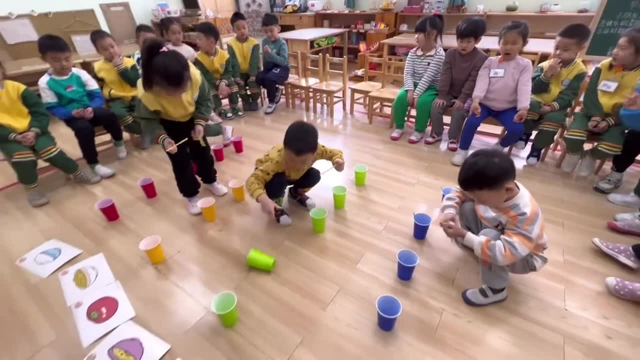 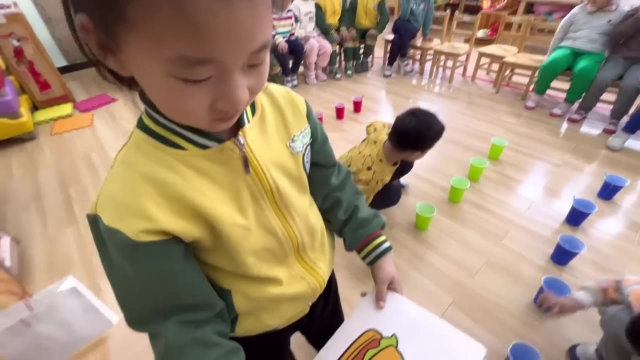 color so you can put the flashcards in front of each lines and the kids have these straws to fill in each cups, one by one. so once they filled up all the cups that they have, they have to go to their flashcards in front of them and say the. 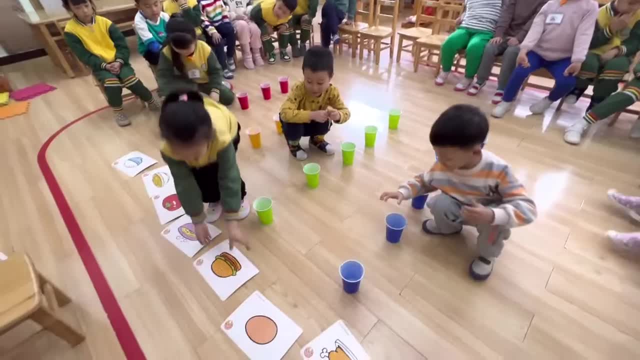 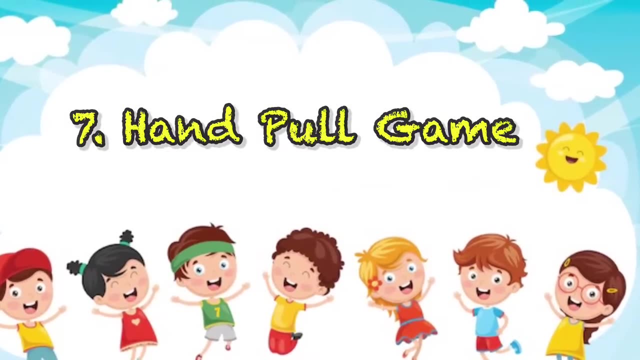 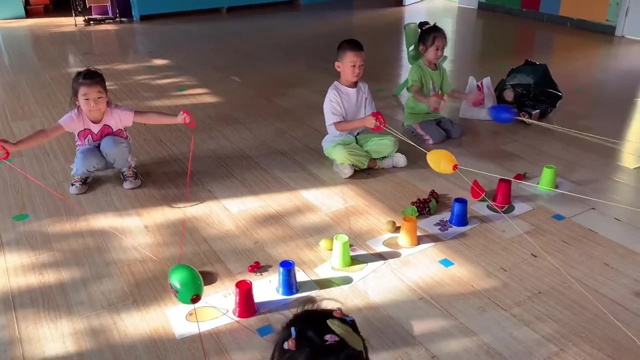 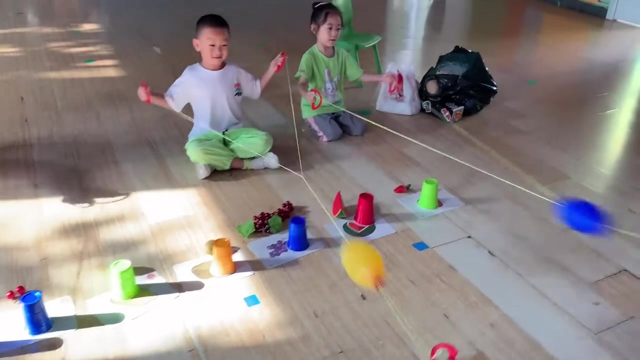 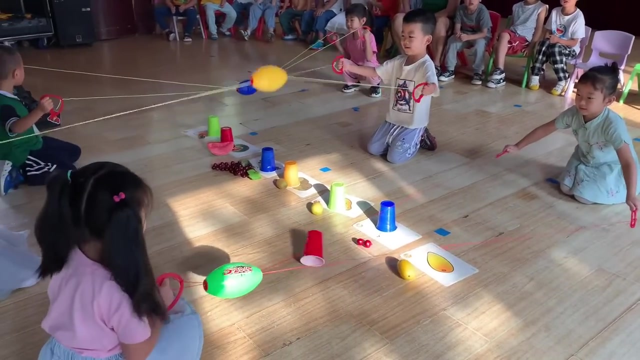 word. what do we have? Hand Pull Game. Hand Pull Game Set. this game is a little challenging or difficult for ages three to four years old, but I've noticed that five to six years old, they didn't have any problem playing this game. So all you have to do is lay down the flashcards between the players and put 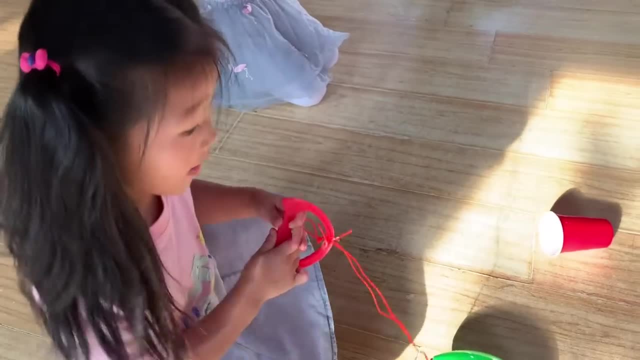 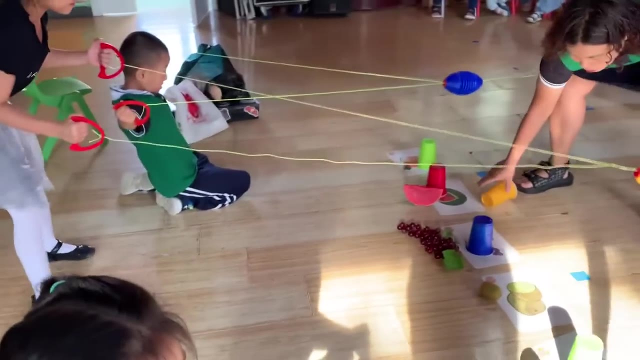 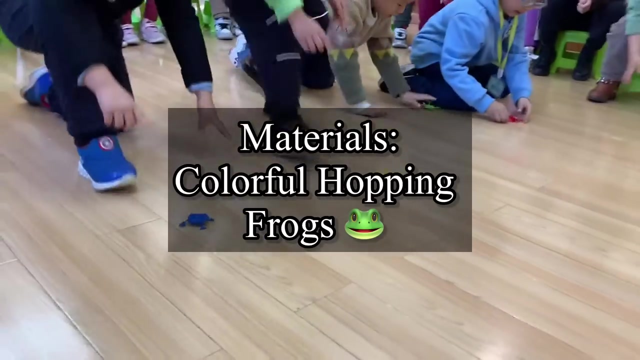 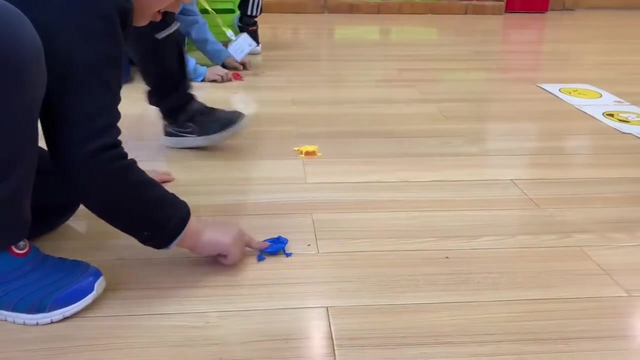 the cups or colorful cups on top of them, and they have to hit the cup and once they hit it, they have to say the word or recite the sentence: hopping frog race materials- colorful hopping frogs. this game is very simple, yet very interesting and fun. beforehand, you need to buy this hopping frogs online and then lay down. 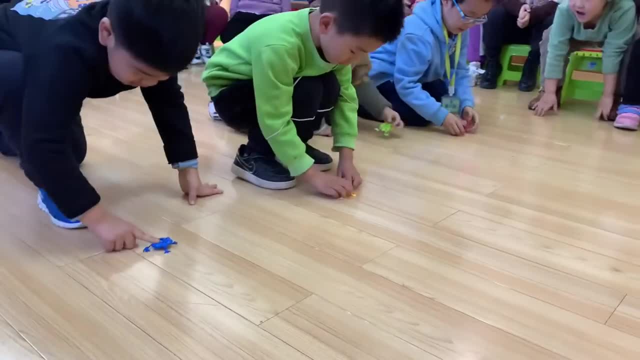 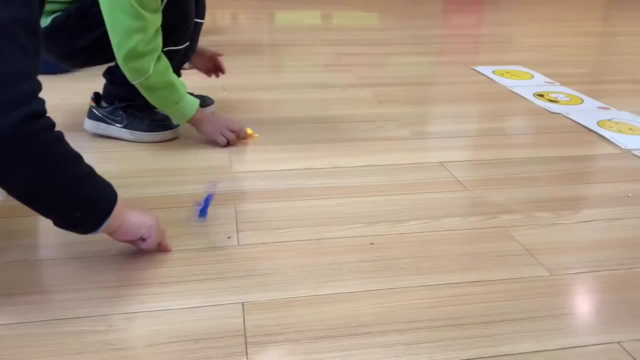 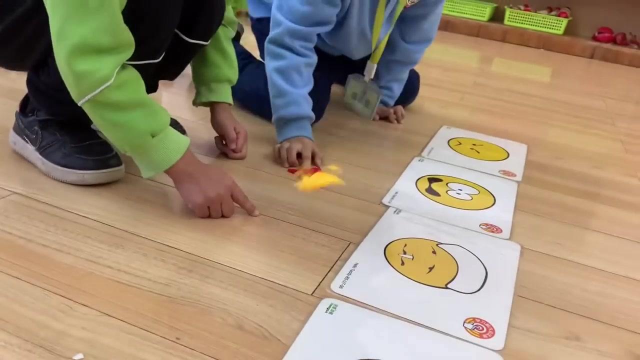 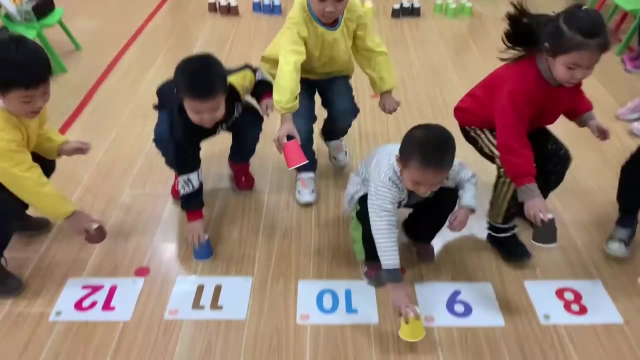 the flashcards opposite to the players. each student will have this colorful frog. they need to press on the back of the frog and then these frogs will jump. they need to race to the flashcards and then say the target words: move the cops, race materials, colorful cups. 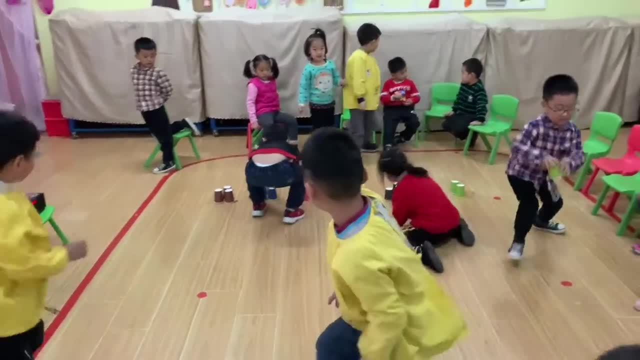 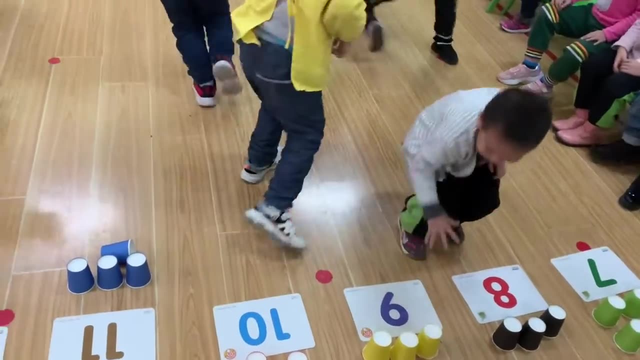 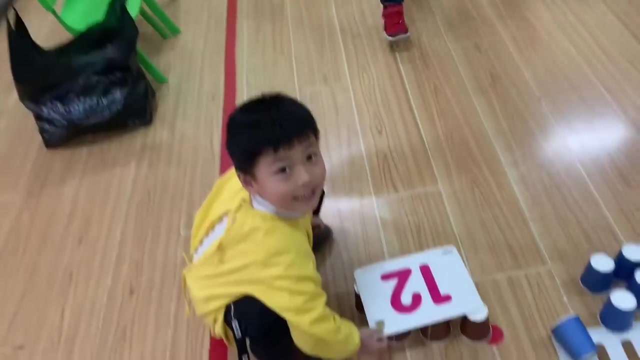 this is one of those games that you need a lot of colorful cups, so what you have to do is lay down the flashcards on the floor and opposite to them are these colorful cups. each player will have to have at least six cups, and they need to. 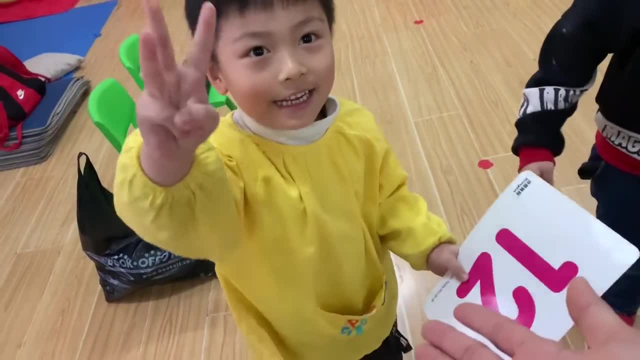 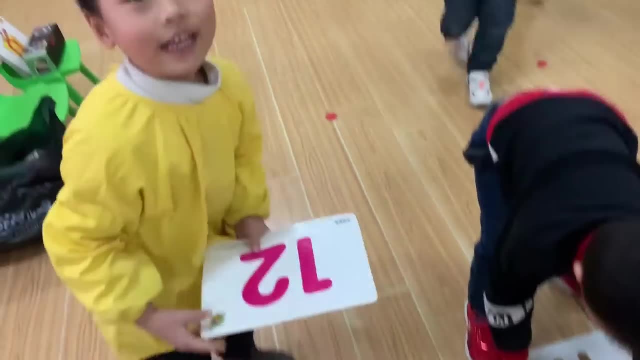 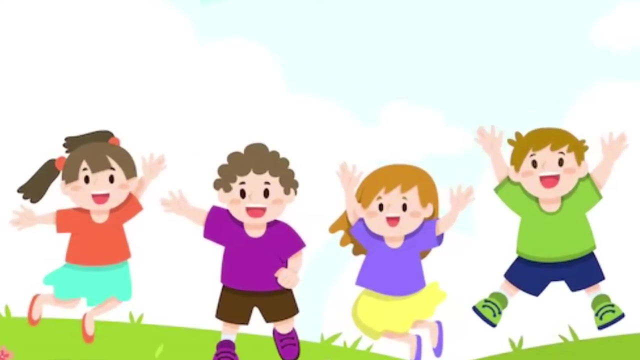 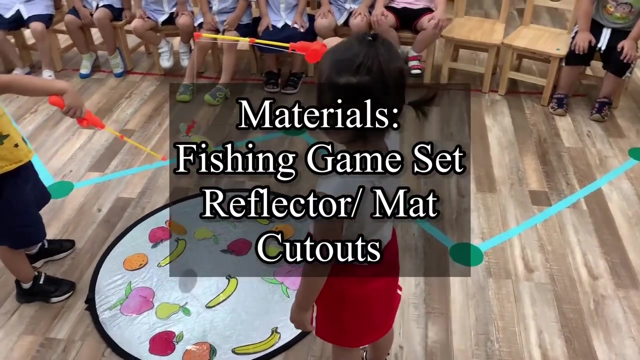 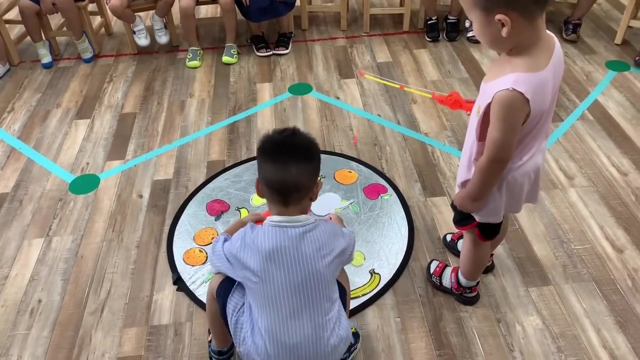 transfer the cup one by one, One by one, to the flashcards and once they have completed all the cups, they have to recite the word. well, fishing game materials, fishing game set reflector or a mat and cat eyes. this game is ideal for ages three to four years old, but it can be played on the 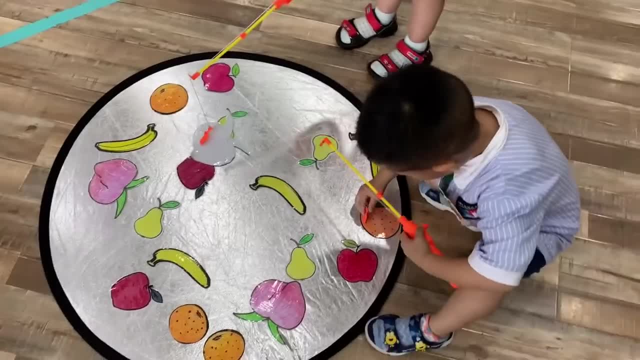 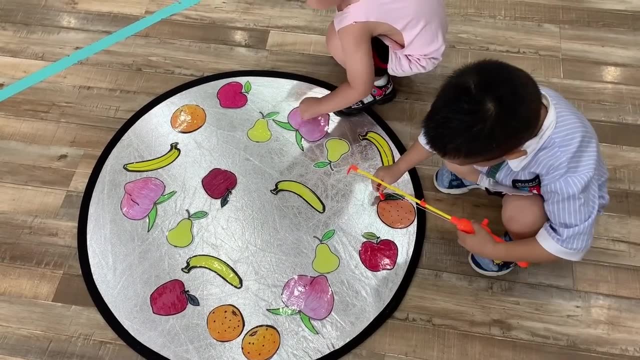 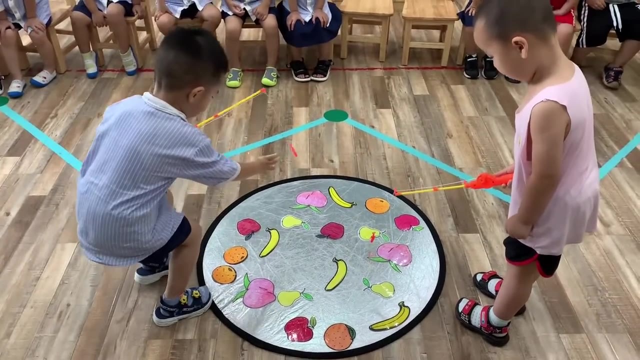 game set the words and can be played also to five to six years old, and all you cat eyes have to do is cut out the target world, for example, in this case, my lesson is about fruits, so I can't talk the fruits and put it on a reflector so that it's 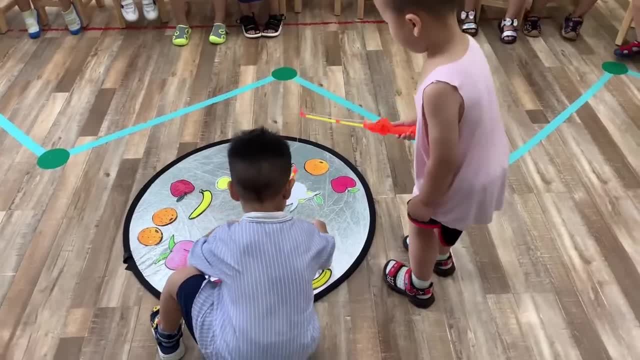 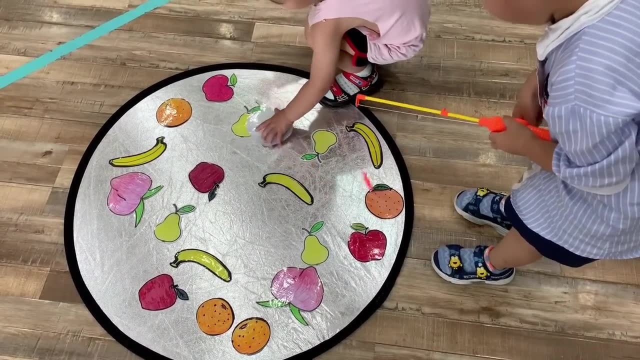 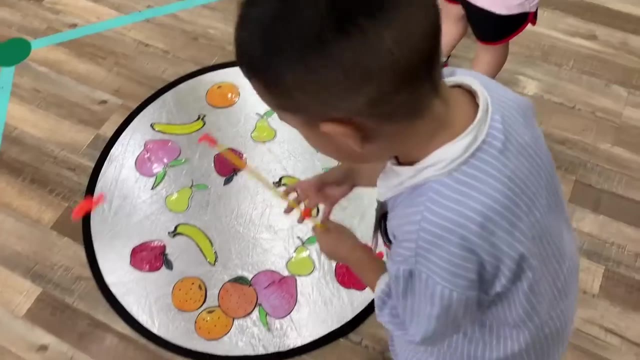 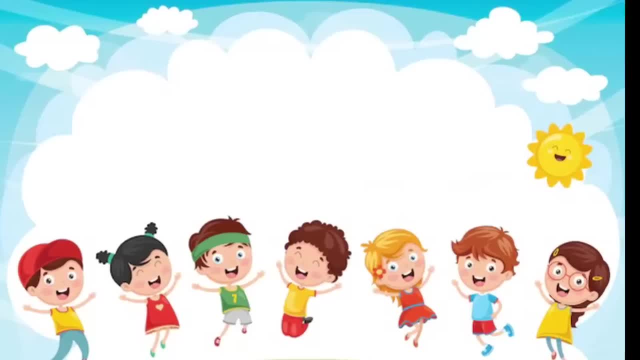 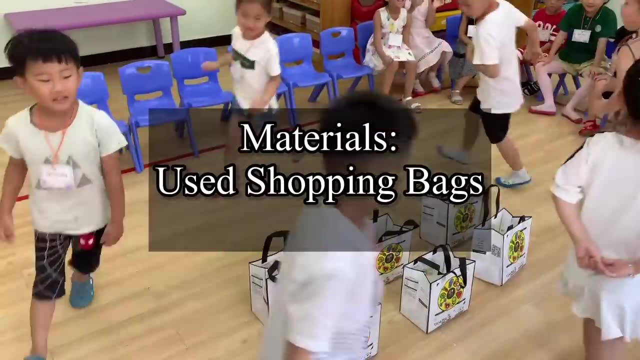 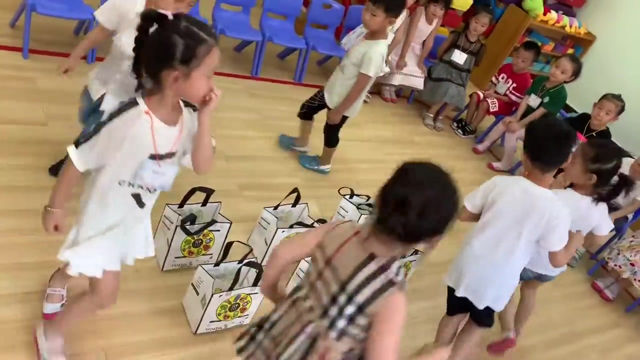 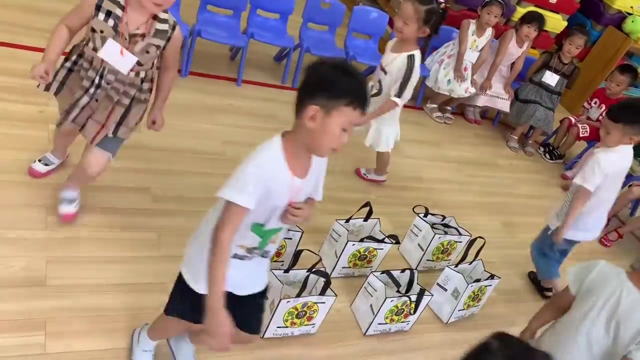 Oh, Go around the shopping bag Materials: used shopping bags. This game is one of those versions of the game trip to Jerusalem. So instead of using chairs, I thought of just you know, using used shopping bags, And then I put the flashcards or target words inside the shopping bags. 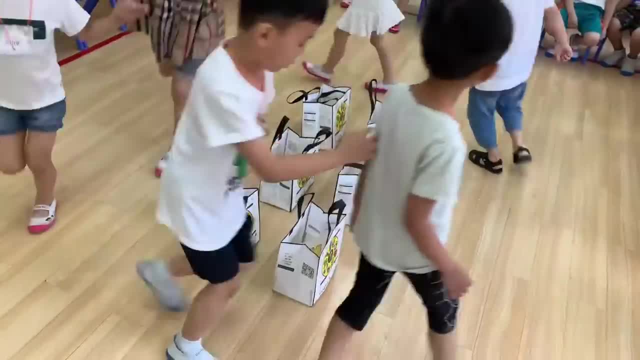 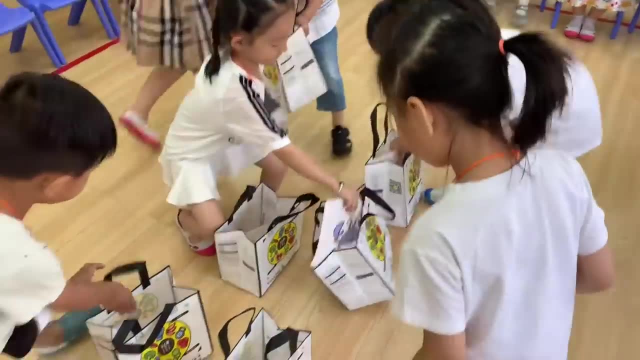 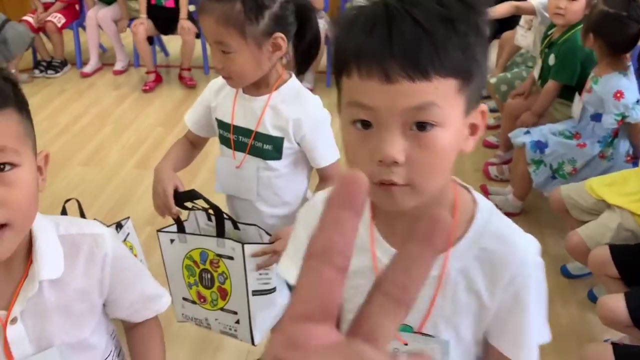 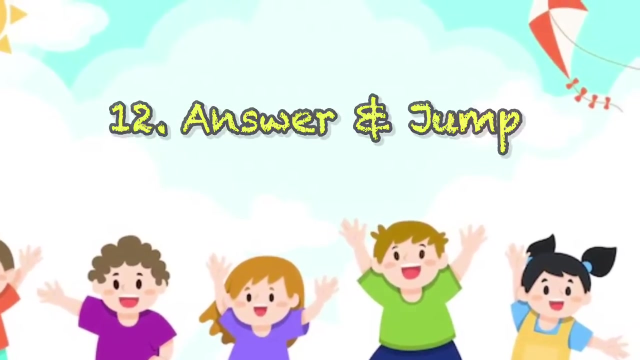 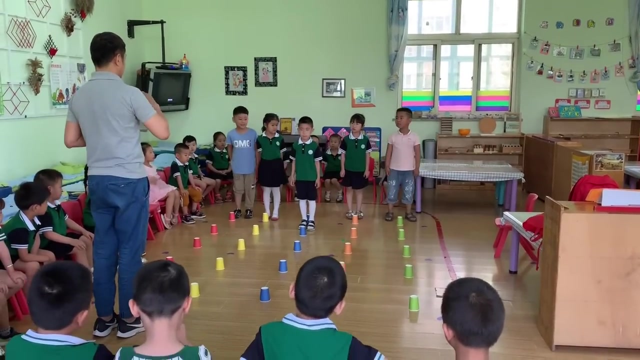 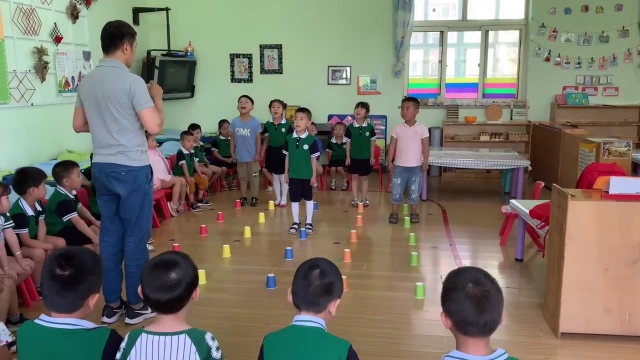 I play the music and Let the kids go around them, and once the music stop They have to choose one of these bags and they have to recite or say the words Answer and jump. Materials: colorful cups. So the mechanic of this game is pretty simple, so I laid on the cups in five lines, according to their colors and 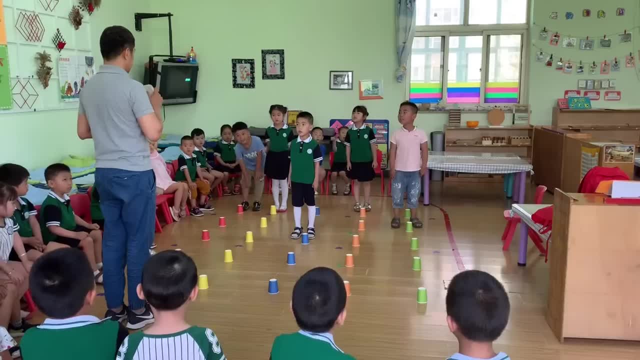 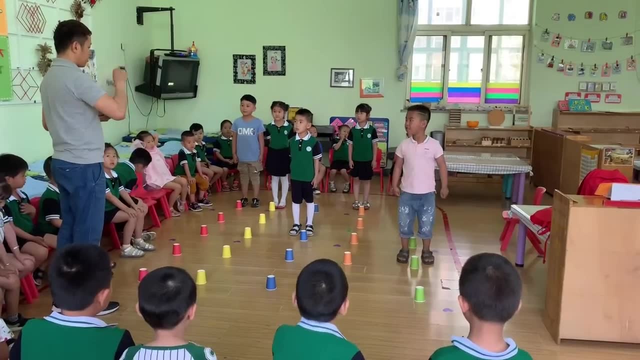 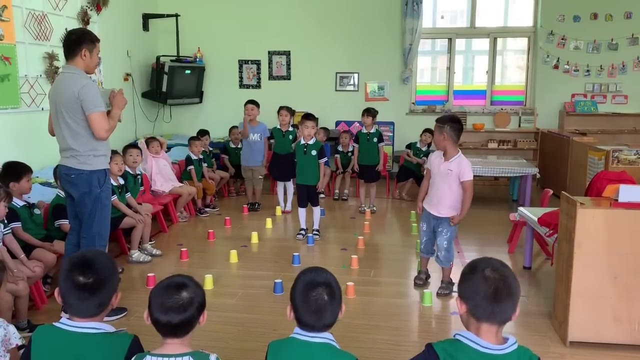 Each student will have a line of cups that they can jump on. So I showed the flashcards or the target words to the children and the first one who could answer correctly can advance by jumping over a cup, and the first one who reaches the finish line wins.